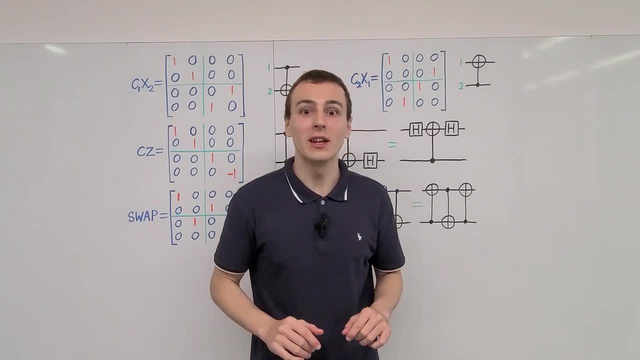 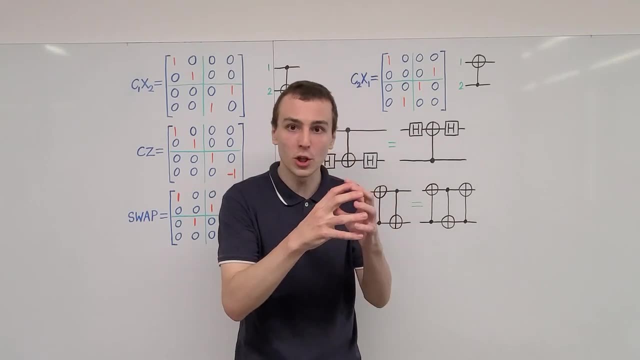 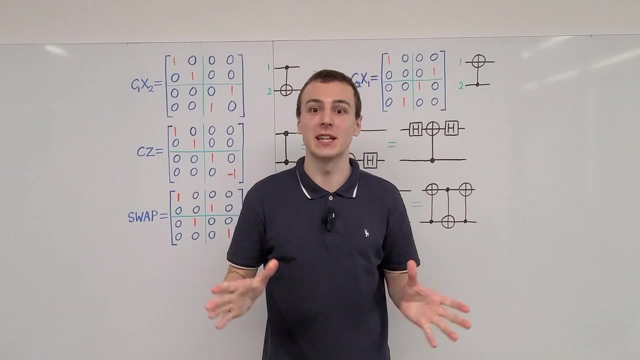 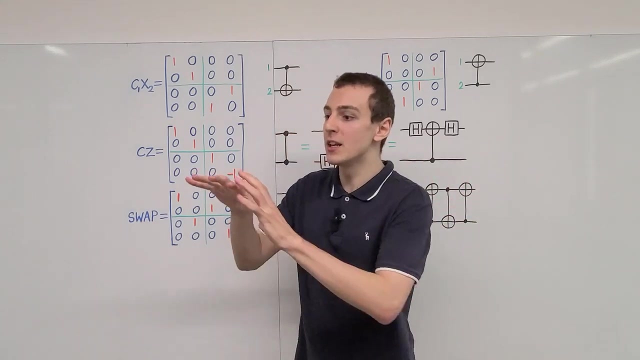 these states as tensor products. For a single-qubit Hilbert space, that is, a two-dimensional Hilbert space, we have two states that are needed to span the entire state and we label those as 0 and 1.. If we consider a single-qubit Hilbert space over here and another single-qubit Hilbert space, 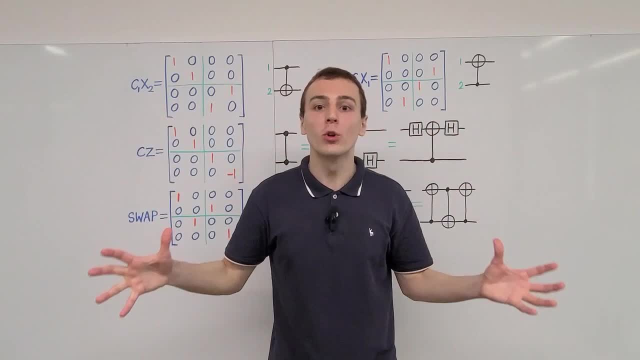 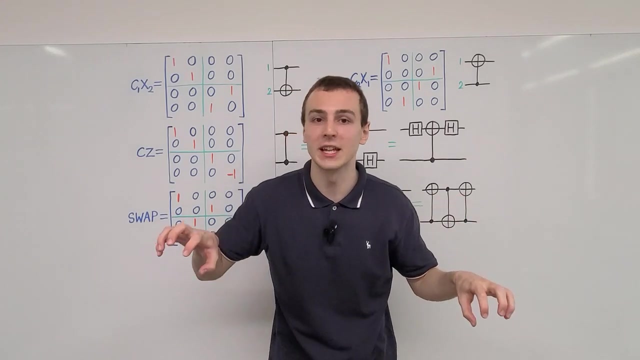 over here. we can combine those into a larger four-dimensional Hilbert space that describes a two-qubit Hilbert space. Now we need four basis vectors to span the entire space. Each of those basis vectors are just tensor products of the basis vectors for the individual single-qubit systems. 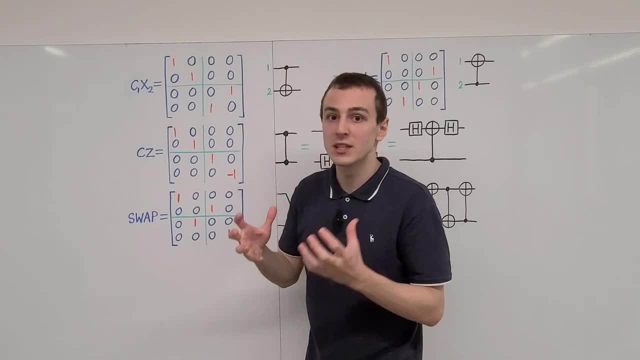 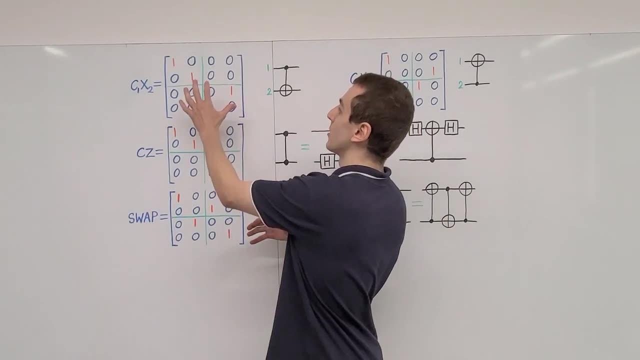 Now we have the computational basis for a two-qubit Hilbert space. What we're going to do is have a look at unitary operators. These matrices over here are unitary operators that act on states. What we're going to do is have a look at unitary operators. These matrices over here are unitary operators that act on states. 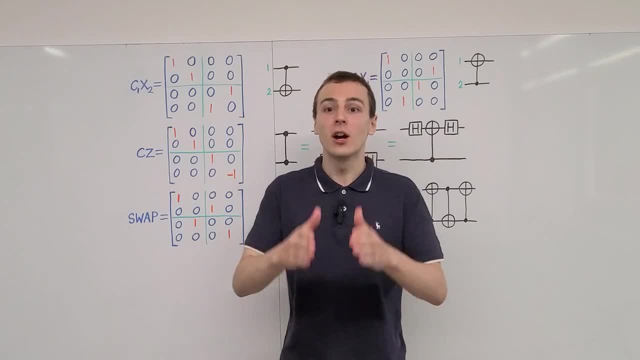 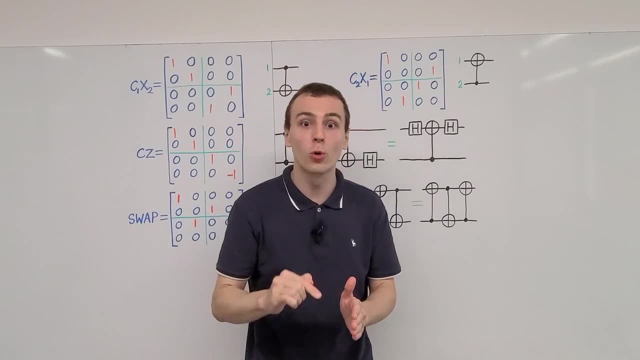 What would the matrix representation of states look like? They would be column vectors. A ket state would be represented as a column vector with four entries, because this is a four-dimensional Hilbert space, and a bra would be represented as a row vector, which. 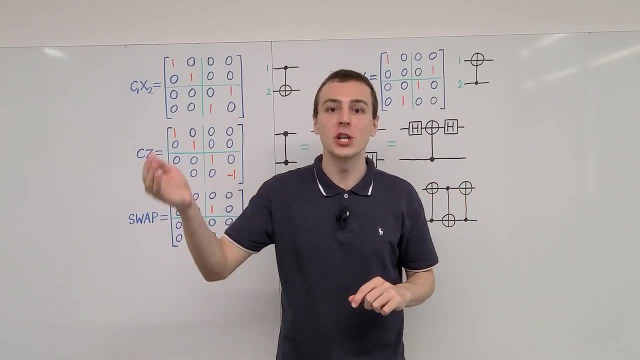 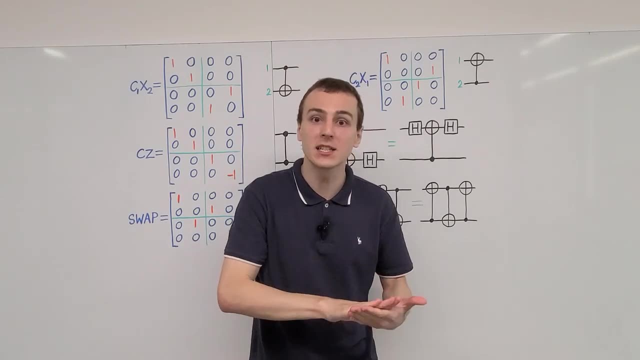 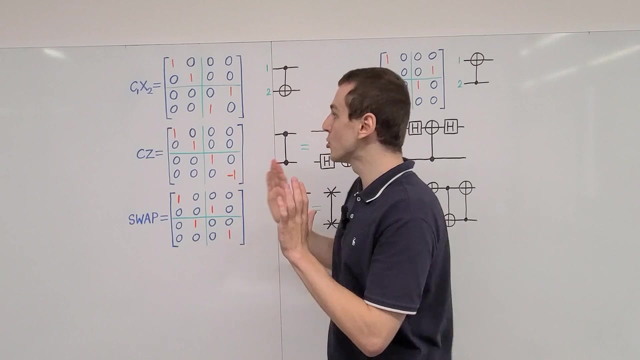 has four entries, but all the entries are complex conjugated. So we take the transpose and we also take the complex conjugate of all of the entries. That's how we go from a ket to a bra In the language of kets and bras. that is Dirac notation. 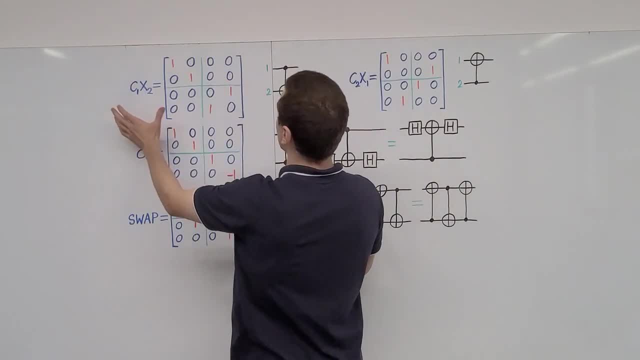 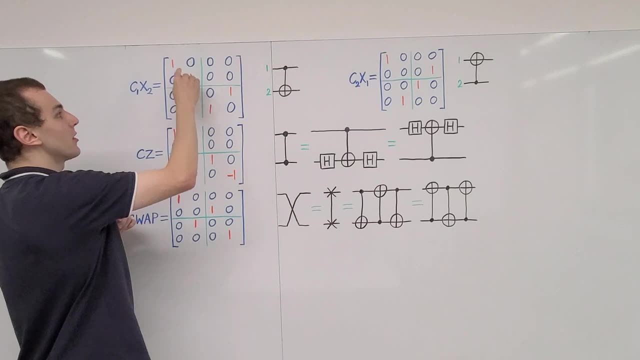 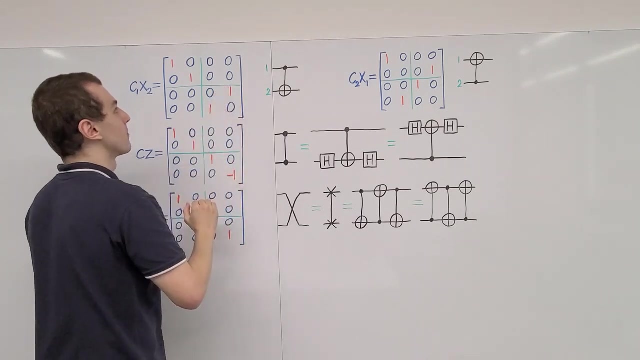 So let's get started by looking at this matrix representation over here. I have conveniently divided this up into four quadrants. You can see that there are only non-zero entries in the top left quadrant and the bottom right quadrant. Over here we can identify the identity. 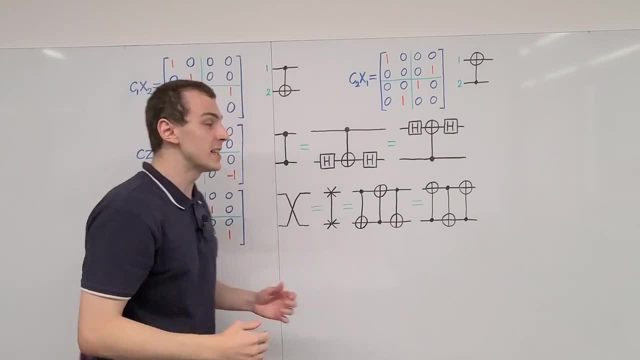 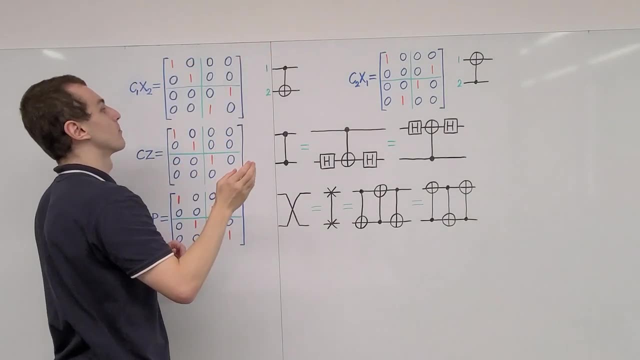 matrix for a single-qubit Hilbert space. This is the two-by-two identity matrix—it has 1s along the diagonal and 0s on the off-diagonal. What about over here? Over here we have the swapped-over version, These two little columns. 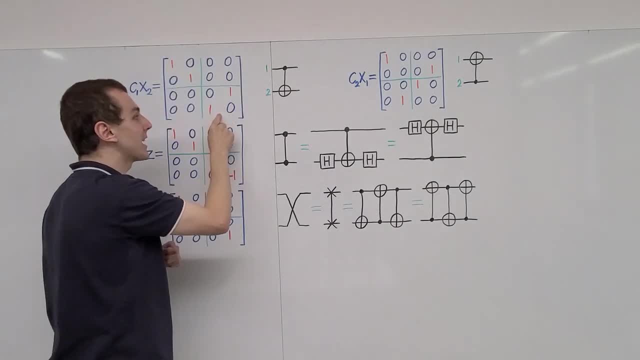 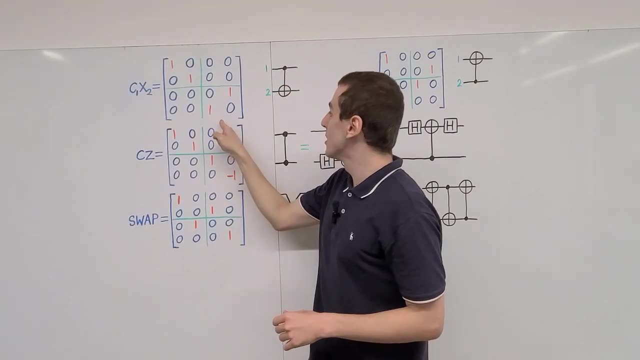 have been swapped around. This is the Pauli x operator, and the Pauli x operator is one of the Pauli matrices. It is analogous to the not-gateune from Boolean algebra and it is sometimes also called the bit flip. When this 2x2 matrix acts on a single qubit state, it has the 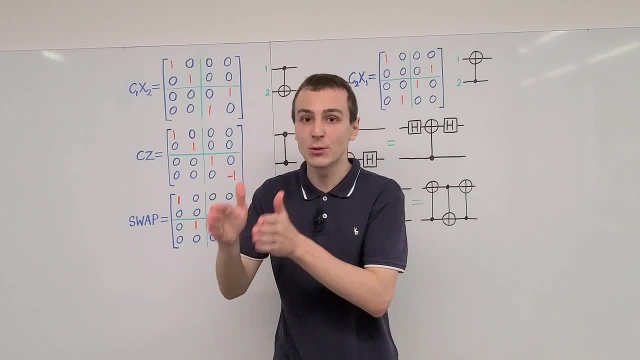 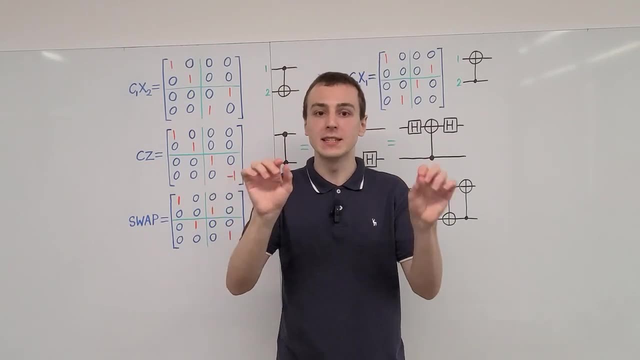 effect of swapping the 0s and the 1s. So the 0 state goes to 1, and the 1 state goes to 0. Always remember that these 0s and 1s on these states are just labels. We could choose any label, but it is convention in quantum. 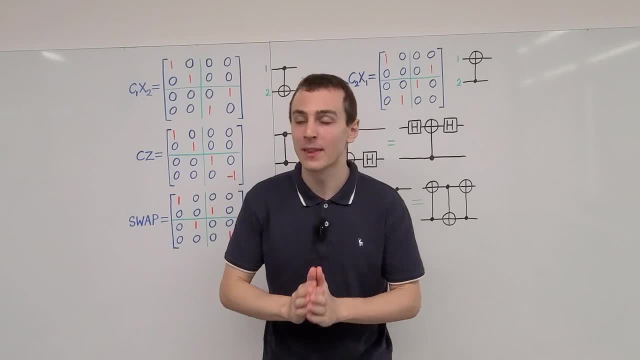 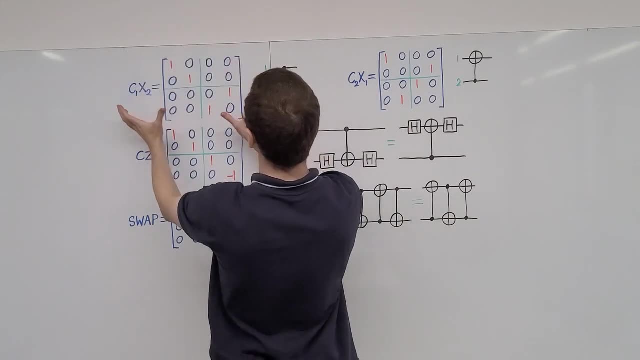 information to choose 0 and 1.. So that is what happens for a single qubit Hilbert space. But what are we dealing with over here? We're dealing with a four-dimensional Hilbert space that describes two qubits And in this special 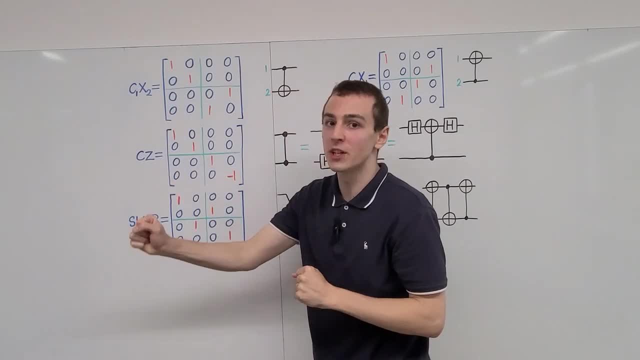 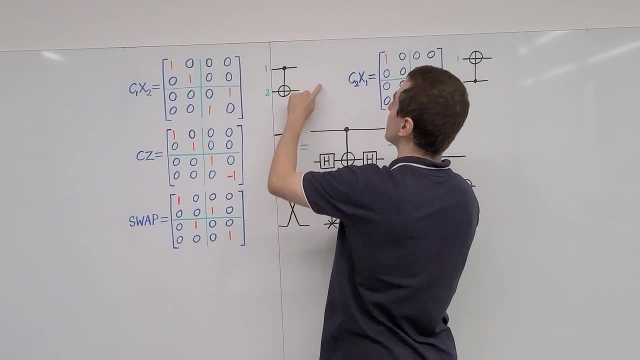 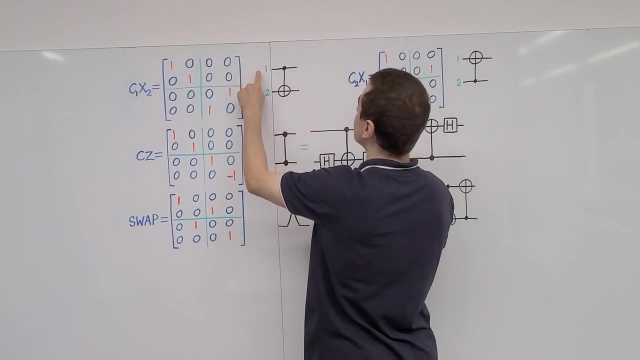 type of unitary transformation. we're actually dealing with a controlled unitary And in particular, we're dealing with a controlled x or controlled 0.. So if we look at this symbolic representation, we see one qubit up over here and another qubit over here. Qubit 1 is acting as the control qubit and 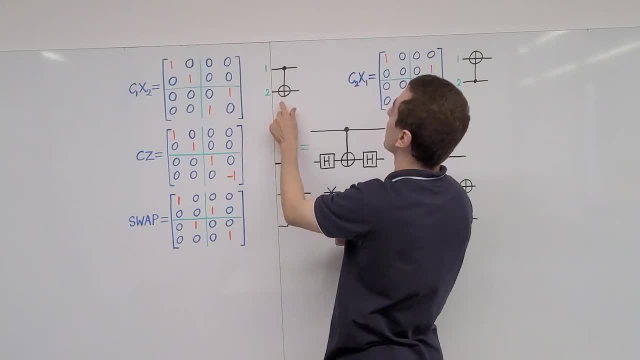 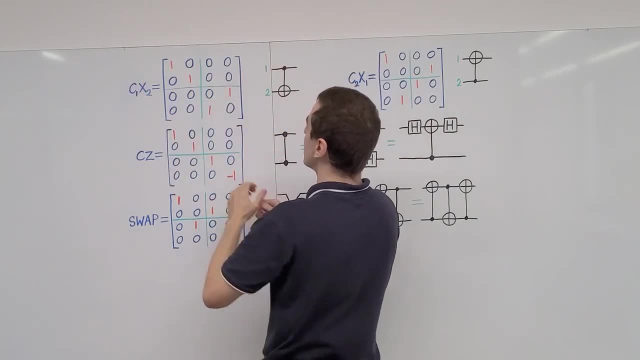 qubit 2 is acting as the control qubit And this symbol is the target qubit. That is what this symbol depicts And this symbol is equivalent to this matrix representation, So this is also called the c0, or the controlled 0, or the controlled x gate, And I have 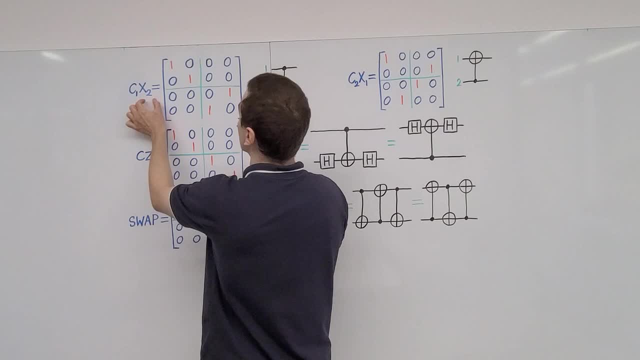 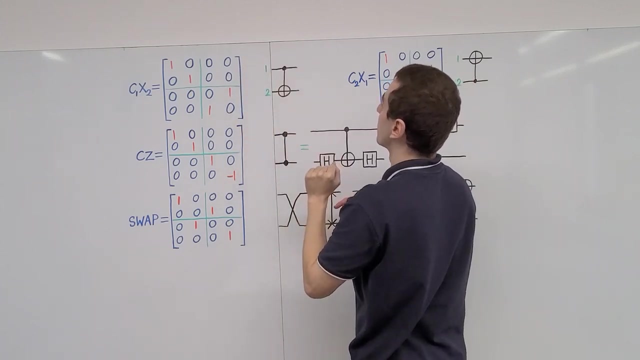 specifically specified these little indices over here where we have 1 and 2.. That is telling us that qubit 1 is acting as the control and qubit 2 is acting as the target. this actually do to a general state of this two qubit system. Well, it will produce, it will have. 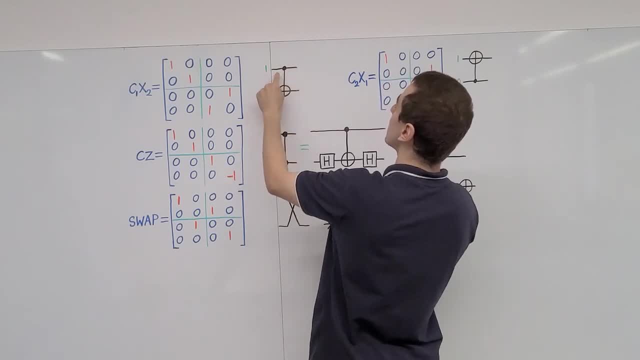 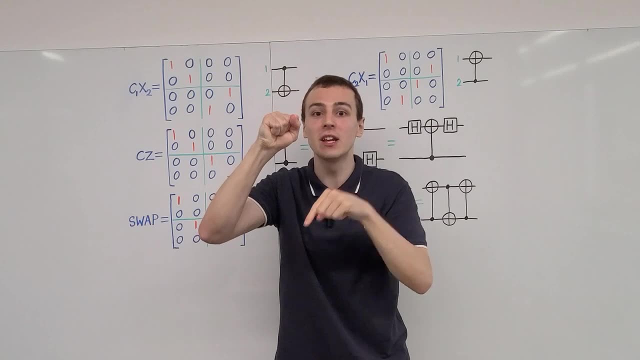 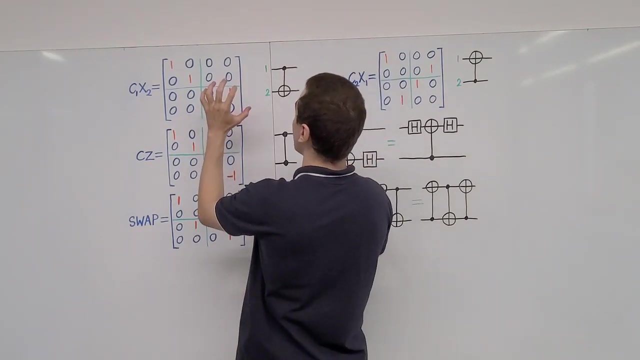 the effect of a NOT gate dependent on the state of the control qubit. So we have a qubit that is controlling the action of another qubit, That is a controlled unitary, And we can actually generalize this and instead of putting a Pali X gate over here, we could put a general unitary. 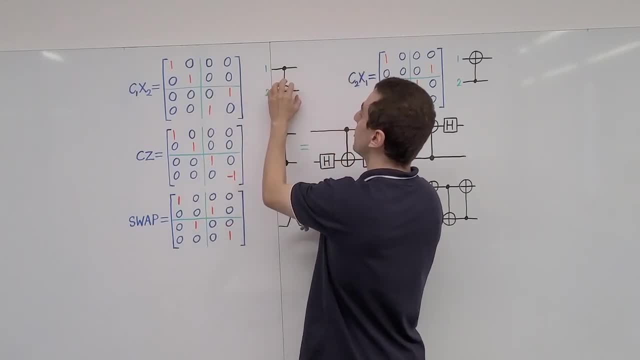 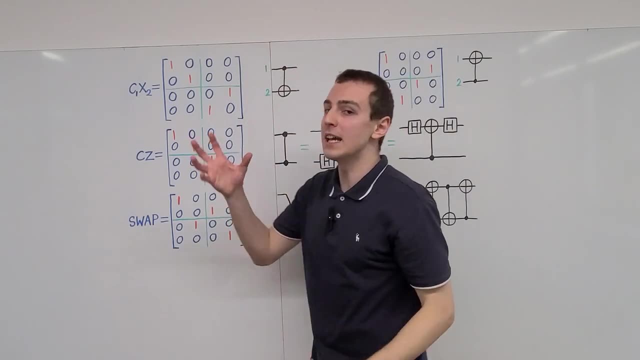 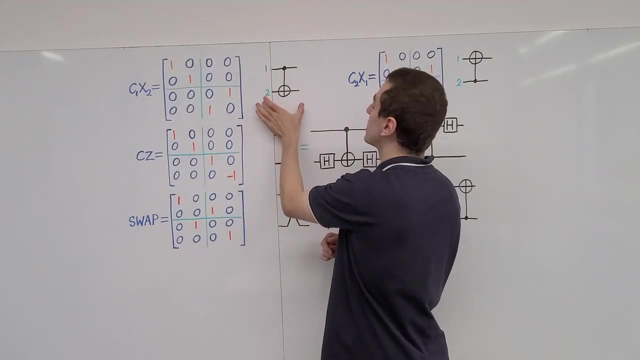 gate. So that would apply this unitary to qubit two, dependent on the state of this control qubit. So that is what is meant by a controlled gate. We have the controlled, NOT gate over here, And this is a very, very important gate in quantum information. We can use this gate to construct. 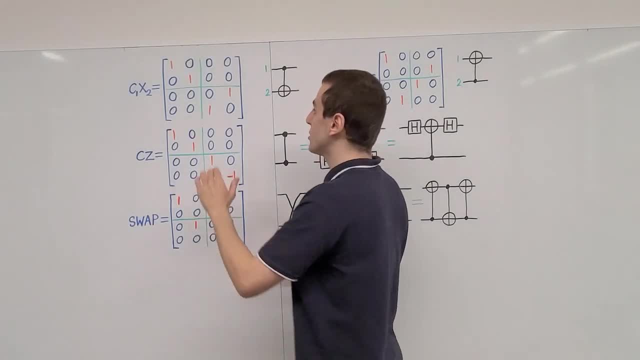 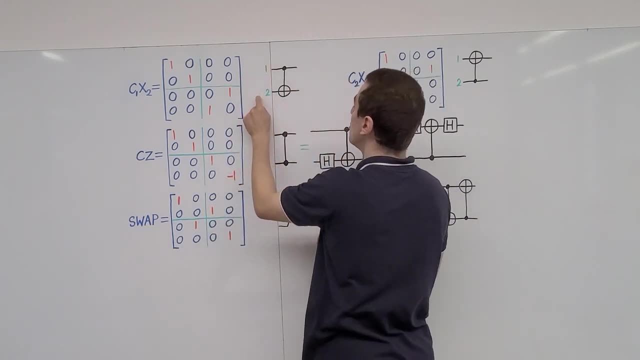 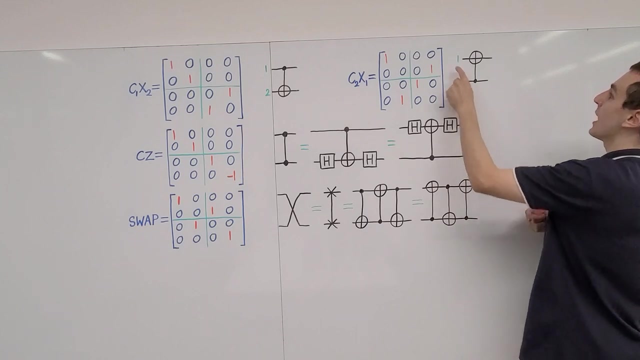 many other useful gates. So this matrix representation is only valid if qubit one is acting as a control gate. So the other gate is actually the control and qubit two is acting as the target. What if we have the reverse? What if we swap the role of these two qubits? Then we would have this diagram over here. 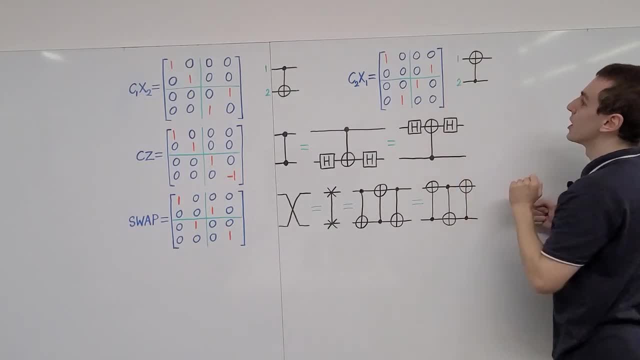 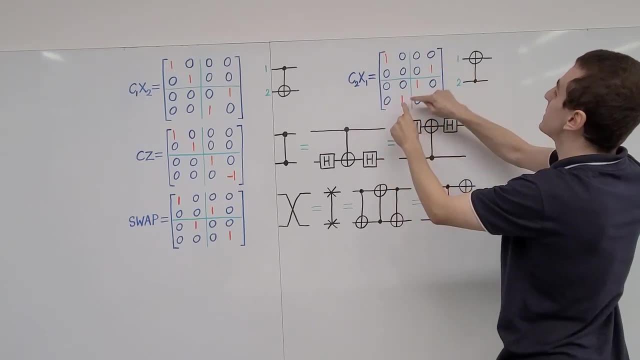 Qubit two is now acting as the control and qubit one is the target. So we have to rearrange the zeros and the ones in this matrix representation. So you can see that now the ones are in slightly different positions to what we had over here. 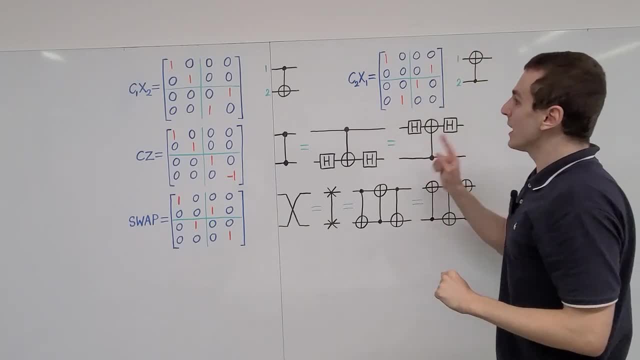 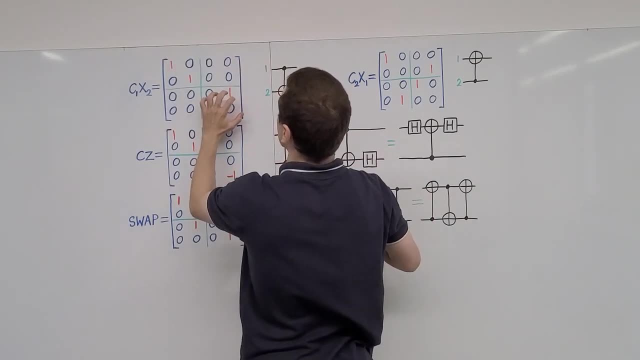 So this is what happens when you swap these guys out around. Now you might think what would happen is you would just swap this quadrant and this quadrant around. You would have a Pauli x up here and an identity down here. That is not what. 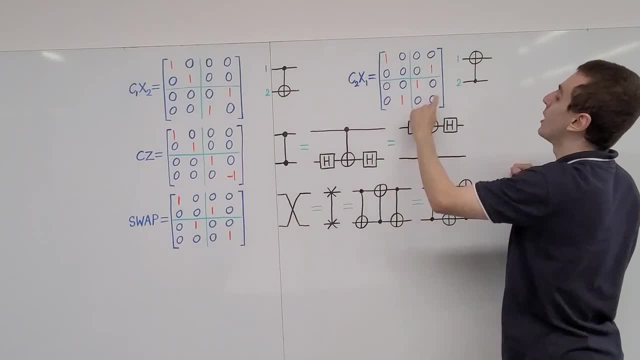 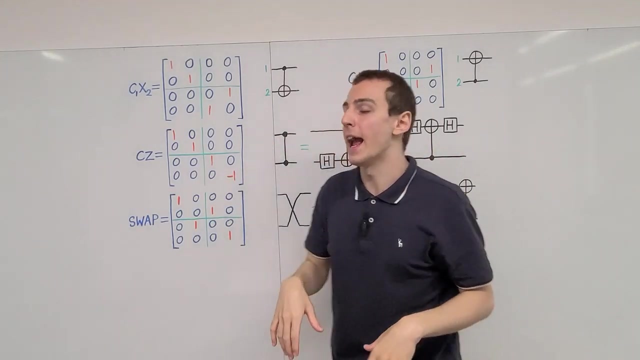 happens? What happens is this rearrangement of ones and zeros, And we will see this in later videos in the quantum mechanics playlist We'll see actually where this comes from. We can define all of these four by four matrices as the sum of Pauli, matrix, tensor products, And that will allow. 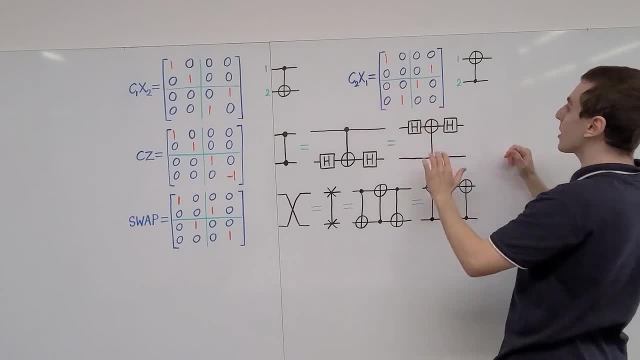 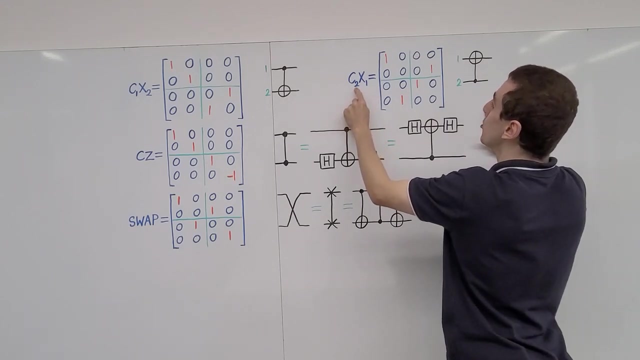 us to clearly see how to construct these matrices. But this video shows us the matrix representations in their form, so we can see what is going on. And we can see that the indices over here in this notation have also been swapped over. This is telling us that qubit two is acting as the 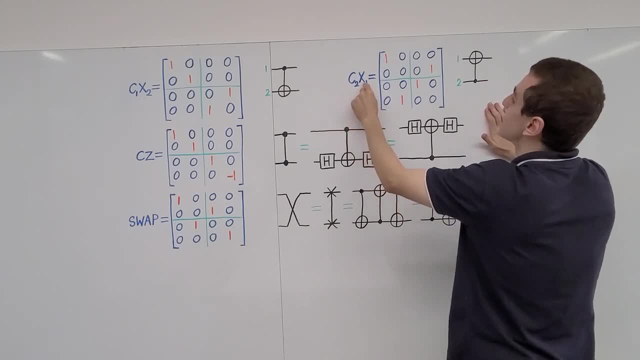 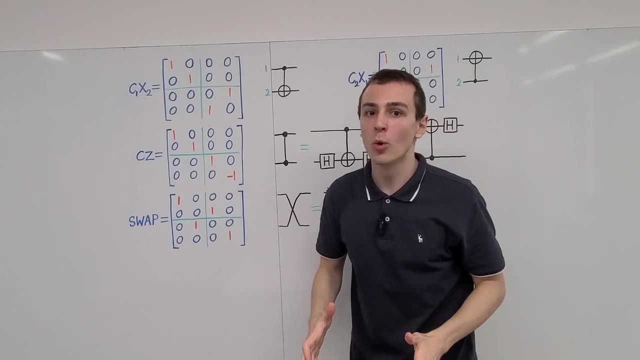 control qubit and qubit one is acting as the target qubit. It is the reverse of what we have over here. So that is the controlled, not gate. We have two of these. We have the control not gate and the target not gate, And we have the. 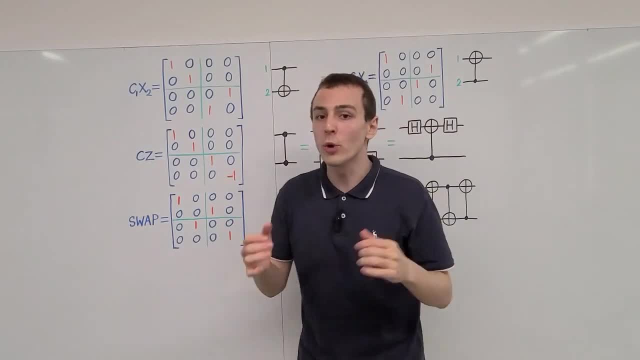 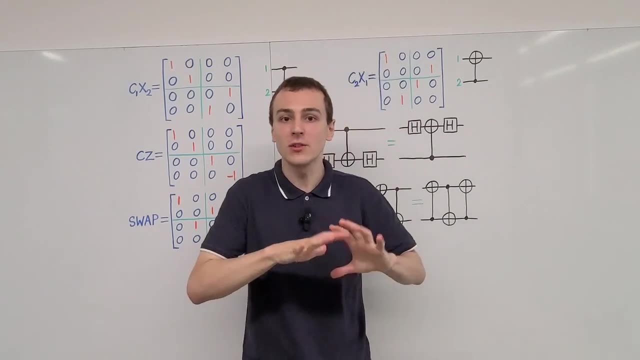 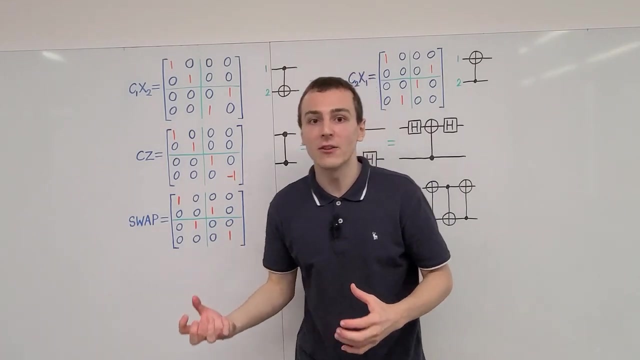 two versions of the controlled, not gate, which change depending on which qubit is acting as the control and which qubit is acting as the target. And, in general, if you have different types of controlled unitaries, the qubit that is being targeted is going to have the effect of that. 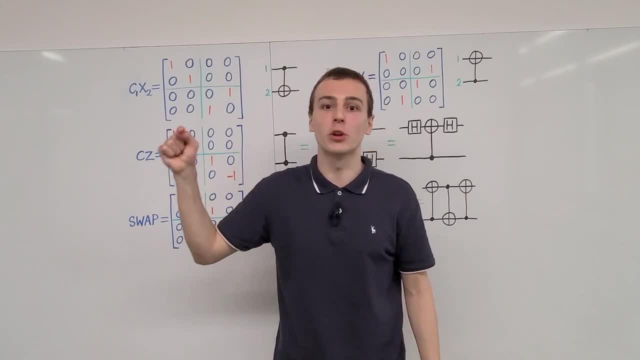 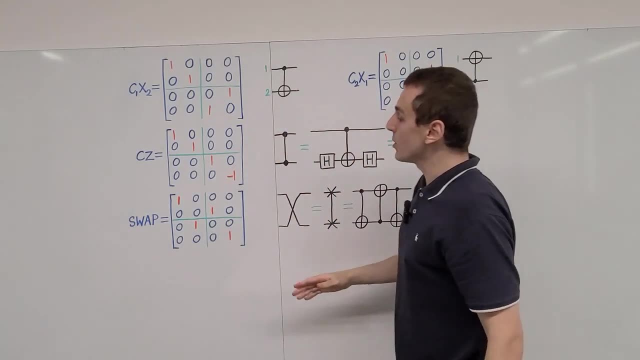 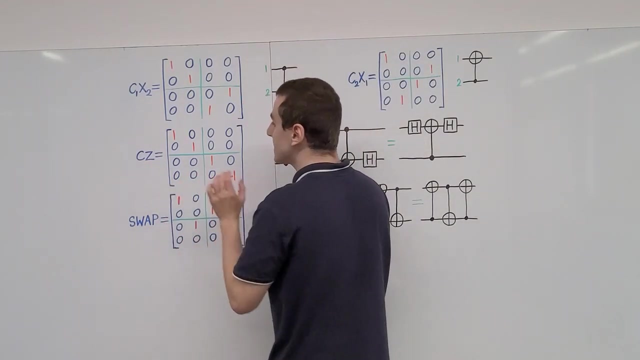 unitary acting on it only dependent on the state of the control qubit. So we're using one qubit to influence another qubit. That is what this gate is actually doing. Let's have a look at another type of controlled unitary transformation, And that is this over here: the controlled Z. This is 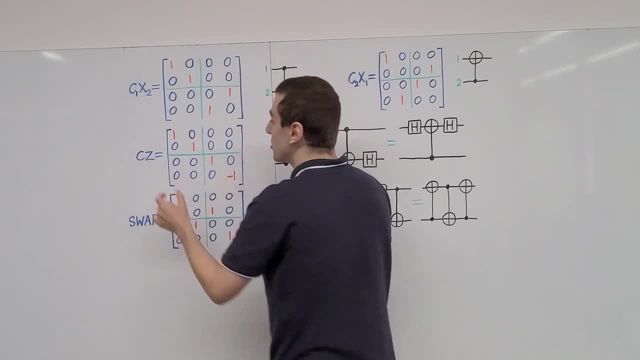 sometimes called the control phase gate, because the Pauli Z operator for a single qubit system is a special case of the phase shift operator. It is a phase shift operator that corresponds to a sine flip. So this minus one over here is actually a special case of a phase factor which is a phase. 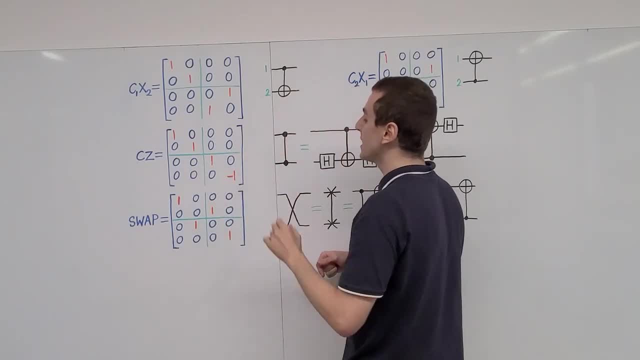 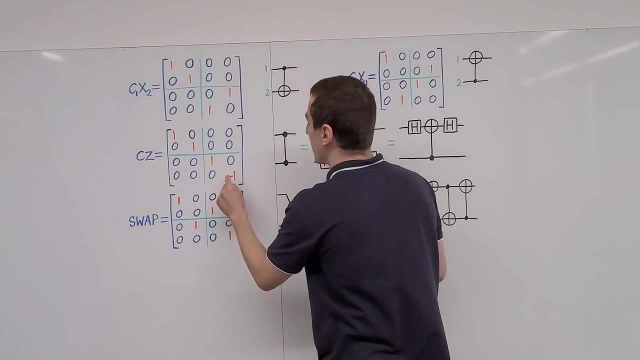 factor which has the form e to the i phi. And if we choose that e to the i phi to be pi or minus pi in the complex exponential, then we will get minus one. So we can choose either plus pi or minus pi. 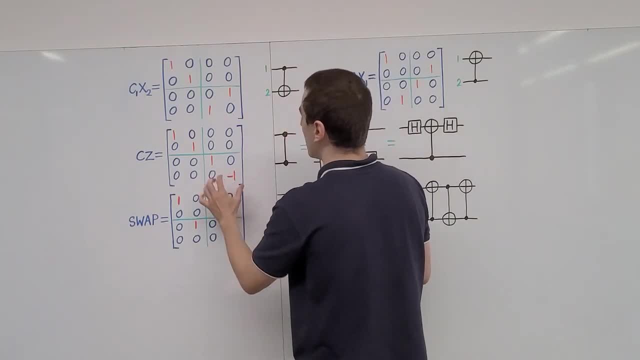 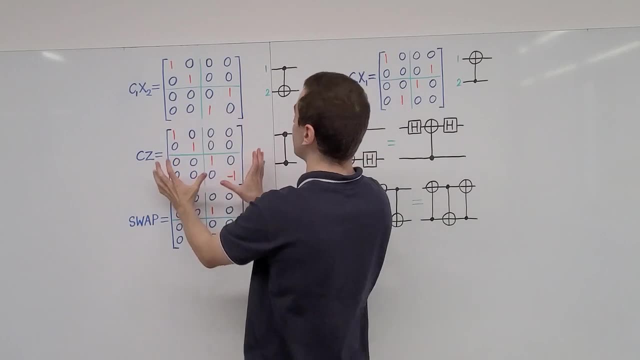 Both are equivalent. They're going to give us minus one over here. So this little quadrant in the bottom right is now the Pauli Z operator. You can see this matrix has the same format that we have up here. We have the identity in the top left. 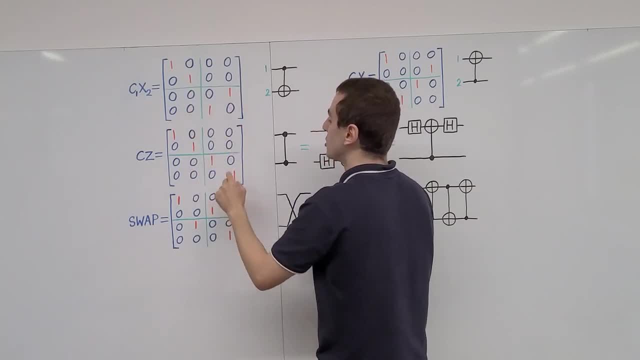 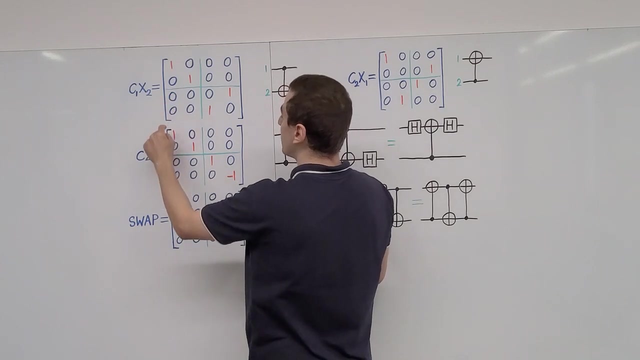 And then a unitary in the bottom right. So what will this do? This will introduce a phase flip. It will flip the sine of the one, one component. So these matrices are constructed with that computational basis. So we can see that this would be zero, zero, zero, one one, zero, one one. 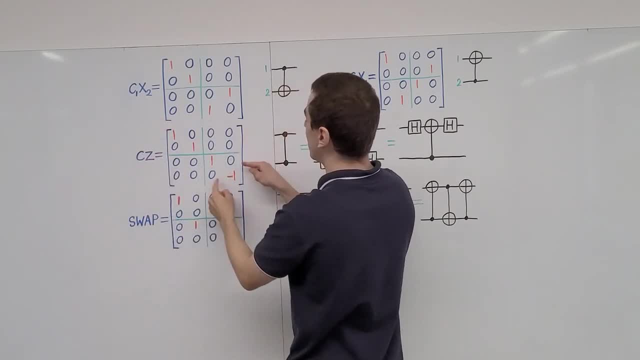 And we have the same thing for the rows and the columns. So this little position over here and this entry in the matrix Corresponds to one one, And that is actually going to tell us that we have to introduce a sine flip. So this sine flip will occur conditional on the state of the control bit. So we have a well I. 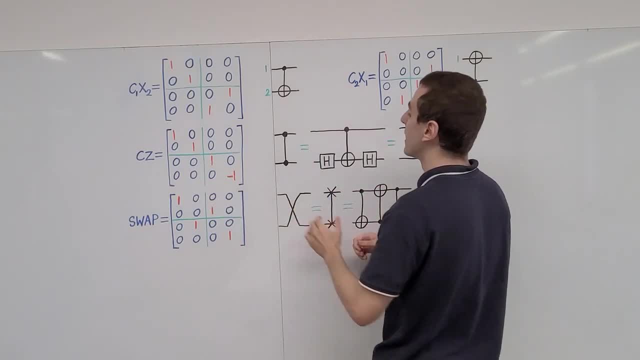 should say qubit. These are quantum analogs of classical bits. This diagram over here represents the CZ gate with a control phase gate. it will introduce that flip dependent on the state of the other qubit. And you can see that it actually doesn't matter which one we call the control and which one we call the target For the control, not gate. 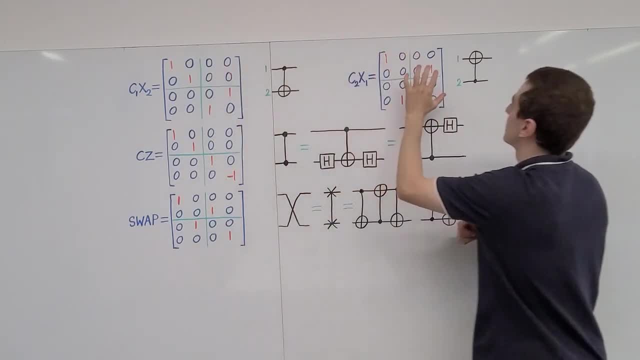 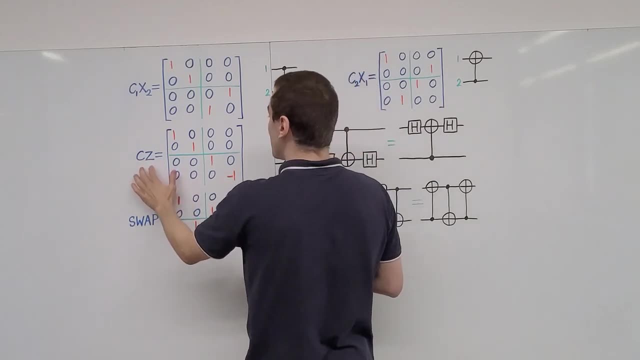 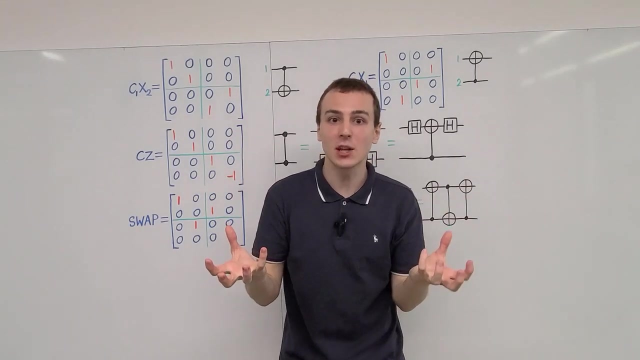 it does matter. This is a different matrix representation for the two cases. If we relabel one and two, we actually have to rearrange the ones, But the control Z gate is a lot more special. It actually is exactly the same If we relabel the states, if we swap the role of the first qubit and the second qubit. 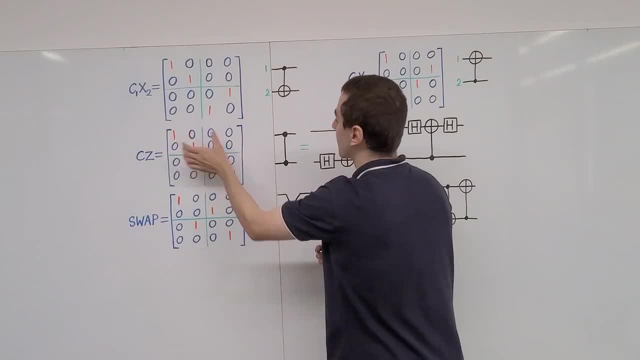 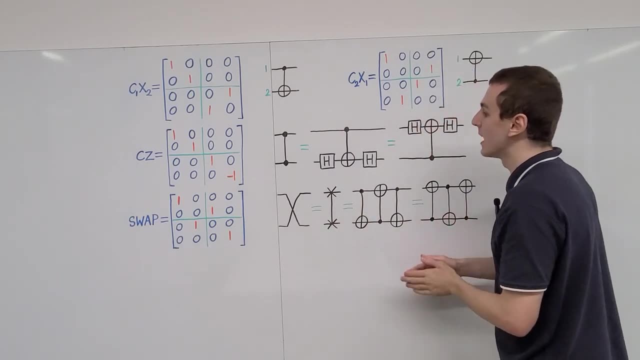 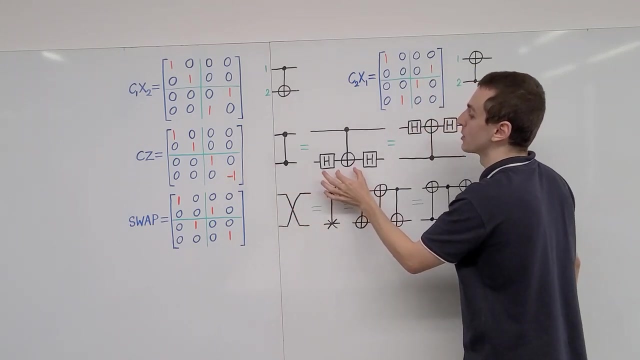 and we switch them around, it will actually be the exact same matrix. So that is why this symbol is used And we will see in the next few videos in the quantum mechanics playlist is that we can actually express the controlled Z gate as a controlled, not gate or control to X gate. If we sandwich that, 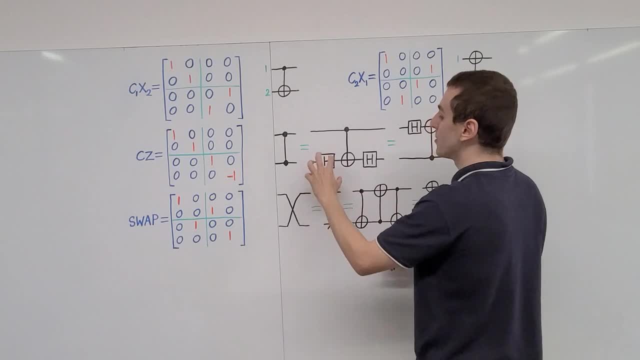 controlled X gate between to Hadamard. so this had a MAR operator and this had a MAR operator are single qubit gates. These guys are only acting on this qubit over here, But this Control Unitary is combining the set of states with a unitary unitary one. 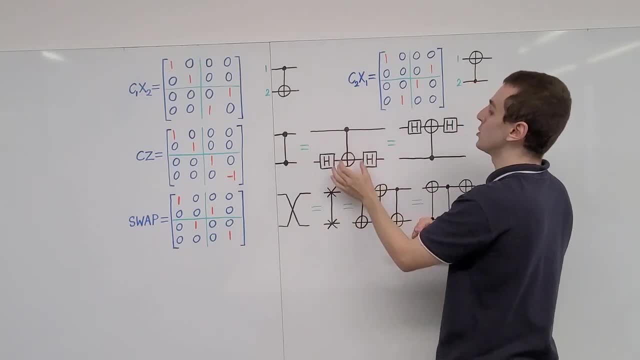 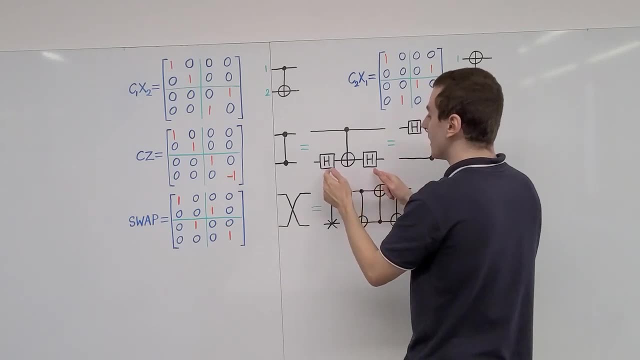 These guys have this central control gate over here, But this controlled unitary, Yeah Well, I guess all it has to do is you. you can pull away this internalっぱ Até. I can't see complete, longest получилось. it's a combined effect on both of these qubits And you can see that, sandwiching something between. 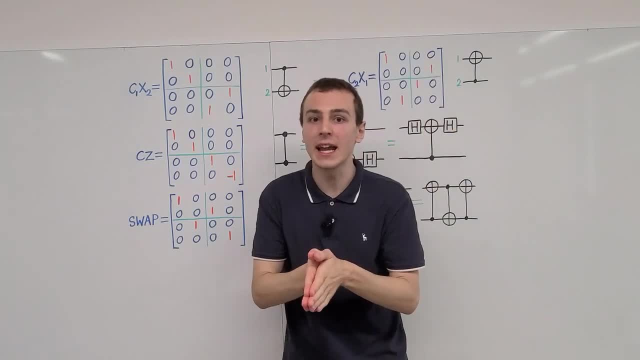 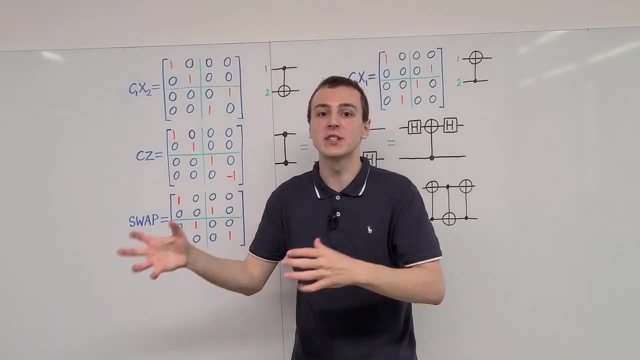 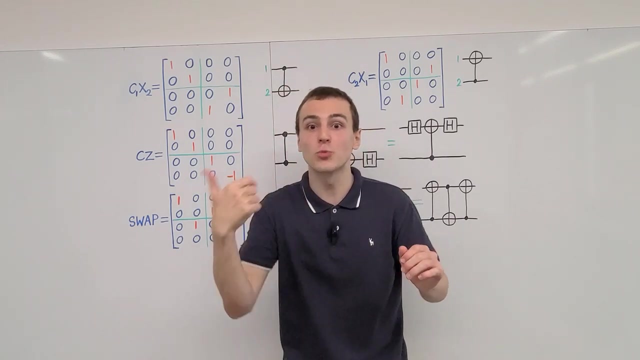 two Hadamards has the effect of swapping the language of phase flips and bit flips. We saw that in some of the single qubit videos and the operators for single qubits. If you sandwich Pali X or Pali Z between two Hadamard gates it has the effect of swapping the two. So Z goes to 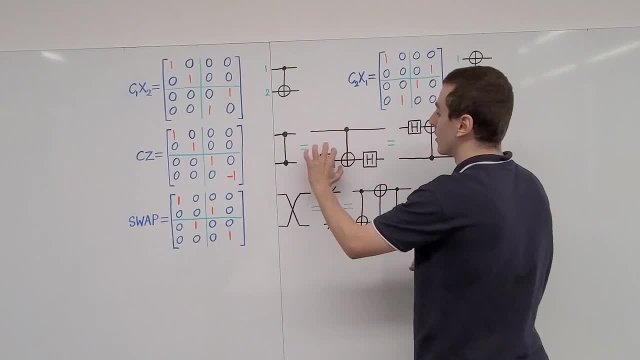 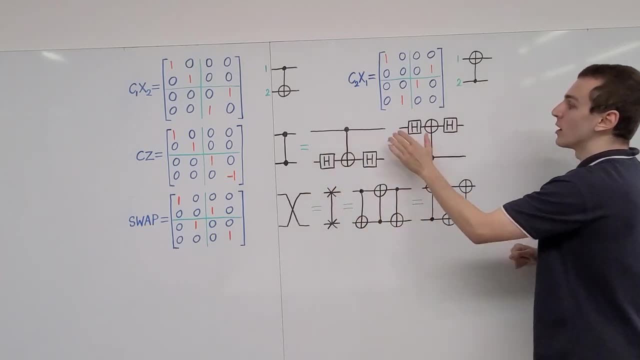 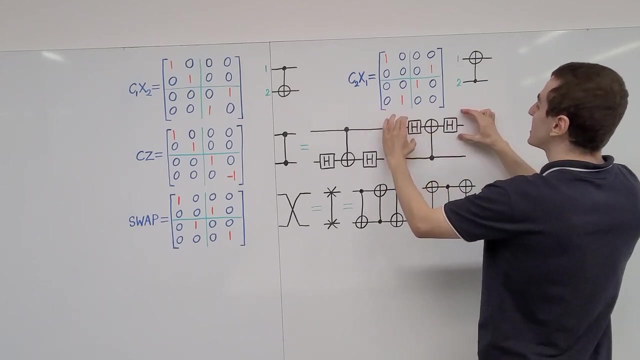 X and X goes to Z. And that is exactly what we're doing over here. We're taking a controlled X and we're turning it into a controlled Z, And we can equivalently do that for this reversed version over here, as long as we apply the Hadamards on this target qubit, So the Hadamards have to. 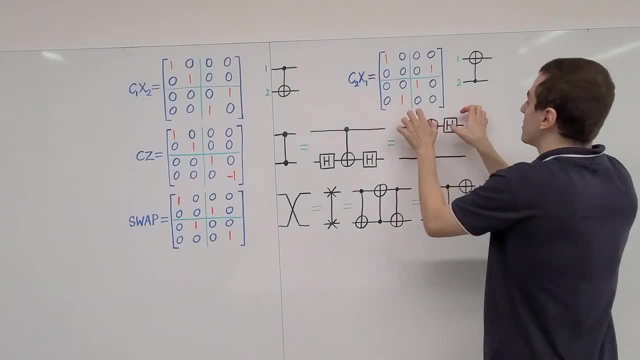 sandwich the target qubit. in order for this to work, You can't just swap the Hadamards and put them wherever they need to be. They have to be exactly here where the target qubit is. So that's our way of controlling the language of phase flips, And that's exactly what we're doing over here. 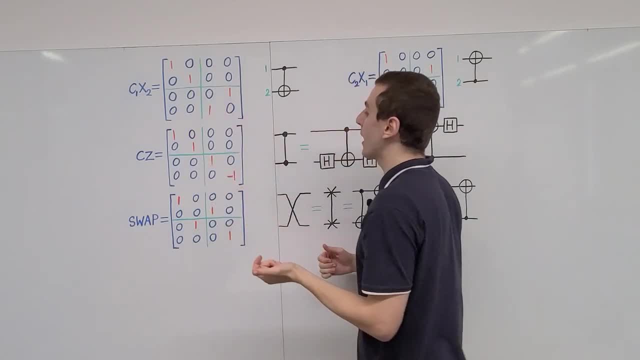 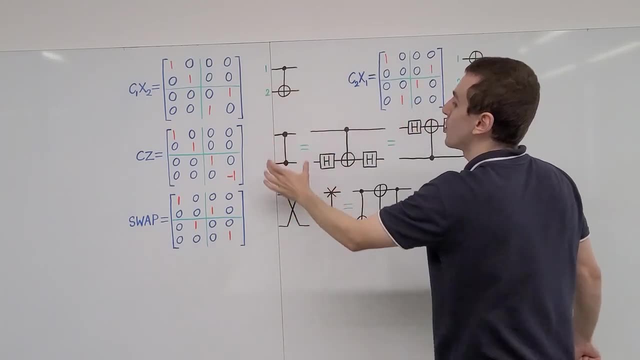 We're converting this X into a Z And we can also go back. We can convert Z to X. So that is why the controlled, NOT gate, is very important, because you can actually use that to construct this controlled phase or controlled Z gate. And these are the schematic diagrams that we would use. 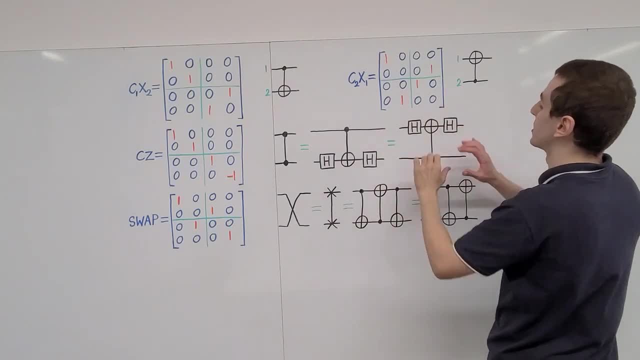 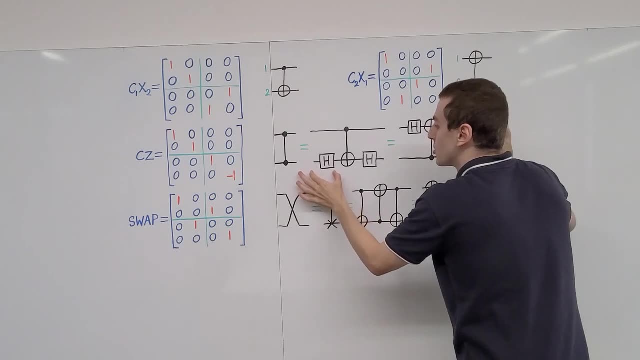 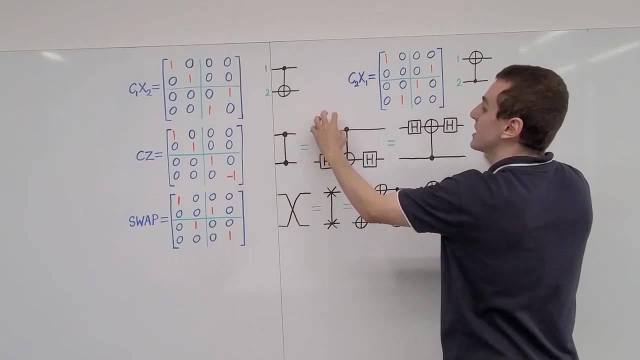 to represent such a transformation or such a circuit, And what would this correspond to in matrix notation? This, over here, the matrix representation of this is a two by two matrix. It is a Hadamard gate, And over here we have the identity, Implicitly we have the identity. 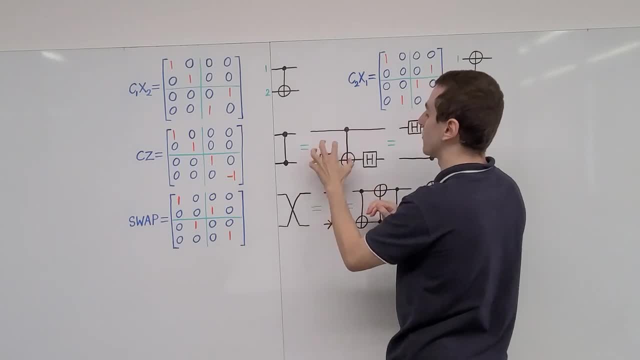 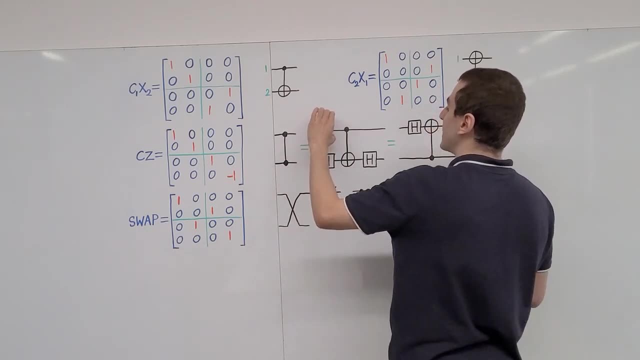 operator over here. So to get a matrix representation for this and for this we would have to take the tensor product of the identity operator with the Hadamard. So we would have identity tensor product Hadamard, identity tensor product Hadamard, And those matrices would sandwich. 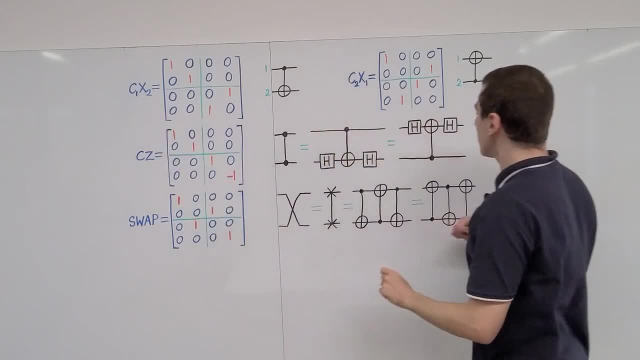 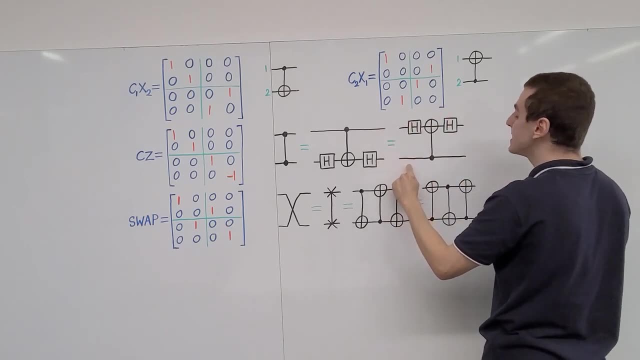 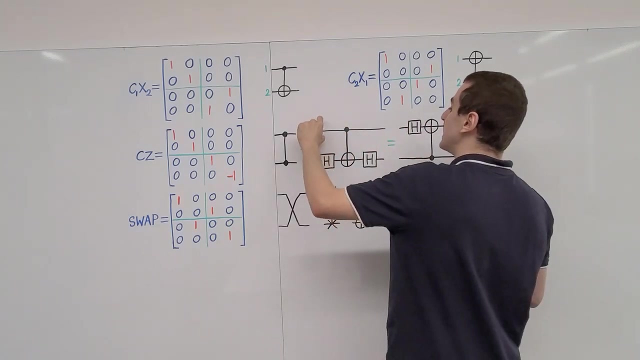 the matrix representation that we have over here. What about this case? We would have to sandwich this matrix representation Between Hadamard tensor product identity and Hadamard tensor product identity. Know that these matrices are not the same. If you take the identity tensor product with the 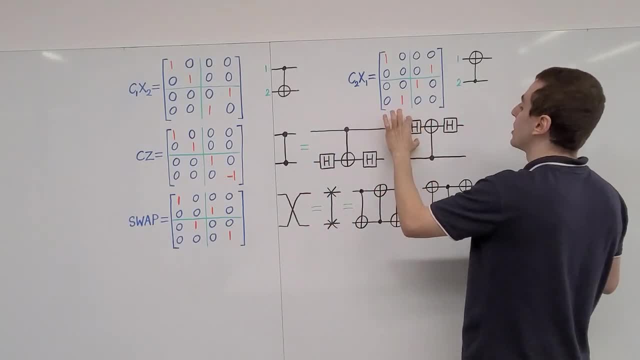 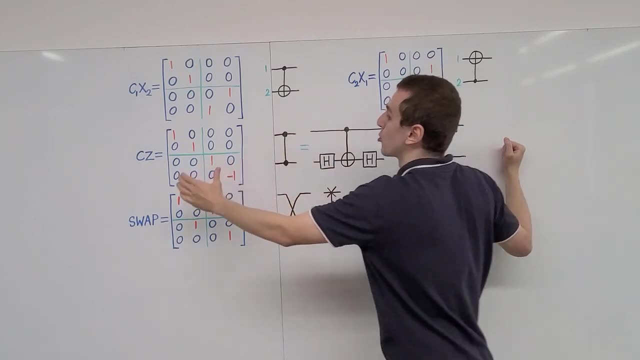 Hadamard. that is a different matrix to if you take the Hadamard and you tensor product with the identity. So this is a slightly different combination but that will give you the exact same controlled Z gate And we will see this. in later videos We will prove why these identities. 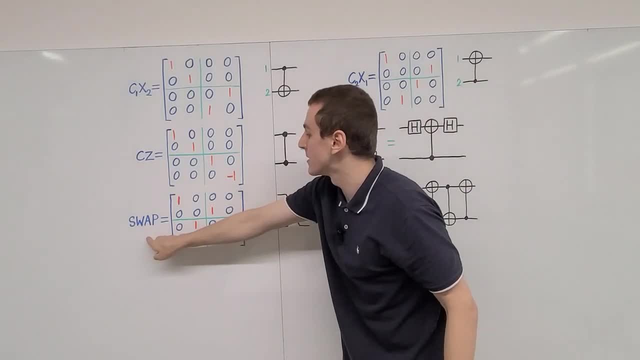 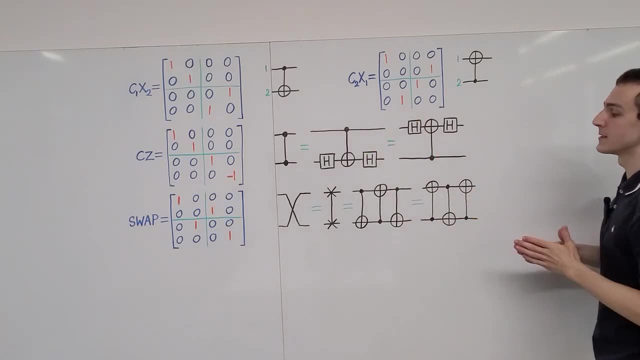 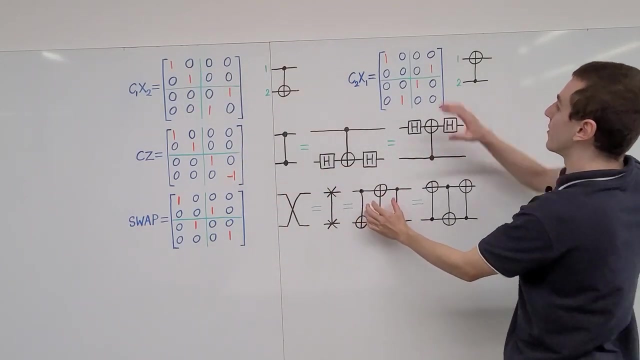 work. Now let's have a look at this swap gate. The swap gate can also be constructed as a sequence of these controlled not gates. If we choose this controlled not gate over here, so that's this matrix- and then we sandwich that this matrix in between two copies of these guys, we will actually get the equivalent. 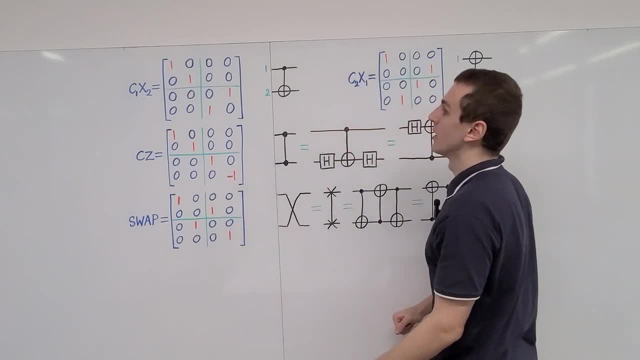 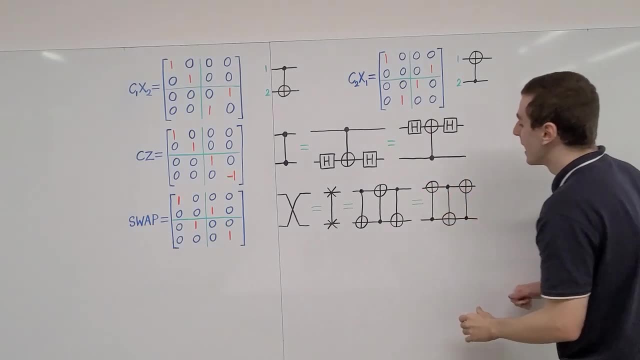 of this matrix over here And you can try this matrix multiplication. try multiplying this by this and then this, Or you could try this combination that will also work. Now, if you do the matrix multiplication, it is a little tedious. There are a lot of entries. 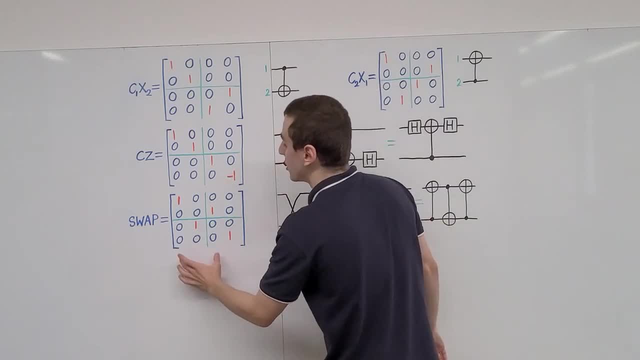 that you have to consider. but eventually you will collapse down to the swap gate And you can see that the swap gate is a little different. It doesn't have that form where we have the identity and then a unitary over here. So it's slightly different because it 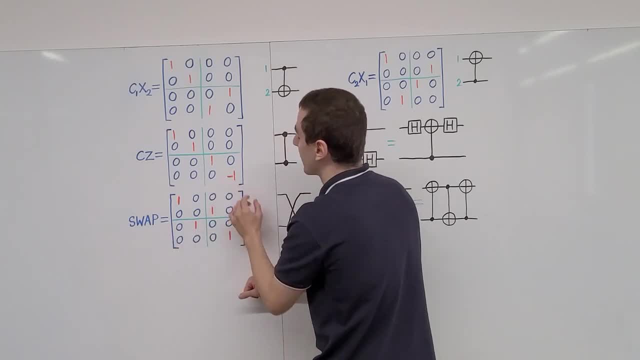 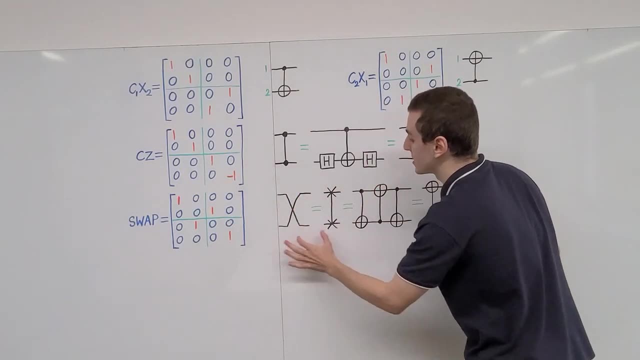 has ones occurring in these quadrants as well, And the effect of the swap gate is to switch information between two qubits, And that is why this symbol and this symbol are sometimes used to visually depict what is going on. So the swap gate can be represented in these. 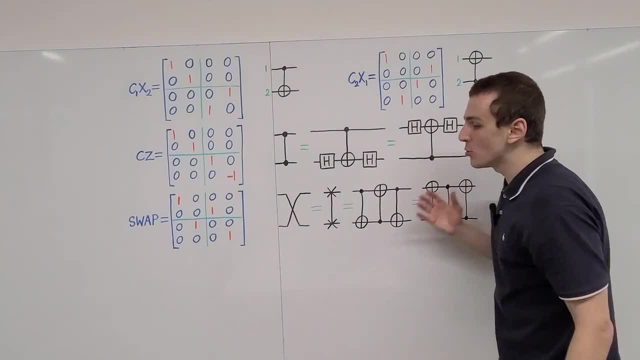 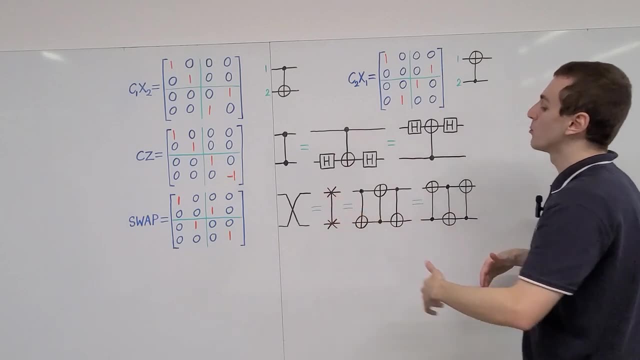 two ways in terms of the controlled not gate, And remember that we don't just have one type of controlled not gate. We have two types of controlled not gate, depending on which qubit is acting as the target and which is acting as the control. So anytime you see, 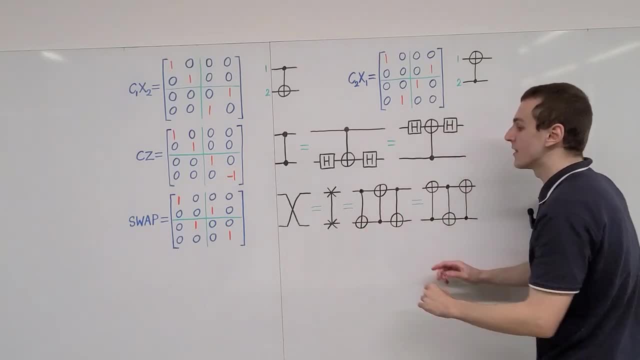 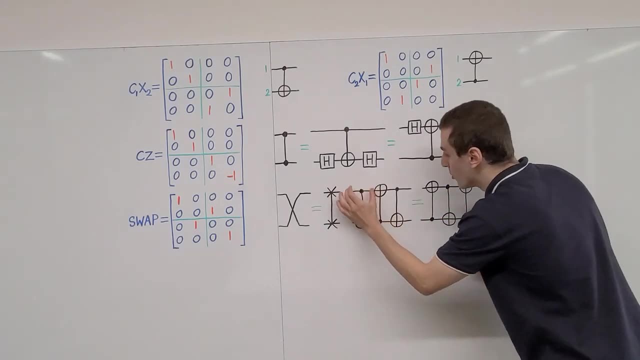 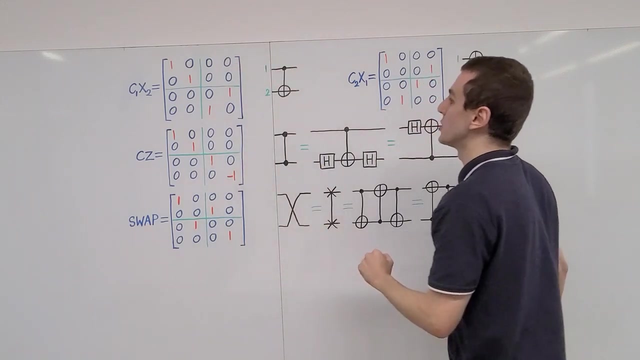 this type of diagram. you need to recognize that all of these guys are just representing matrices. So you can also write this in the language of matrices And if you have a sequence of these gates that you're applying to several qubits, you can represent them as matrix multiplication. You first apply this matrix, then another. 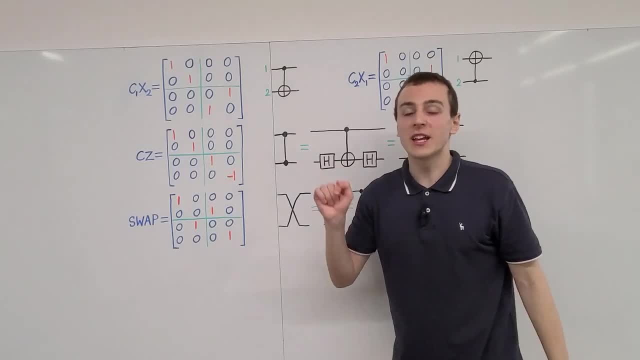 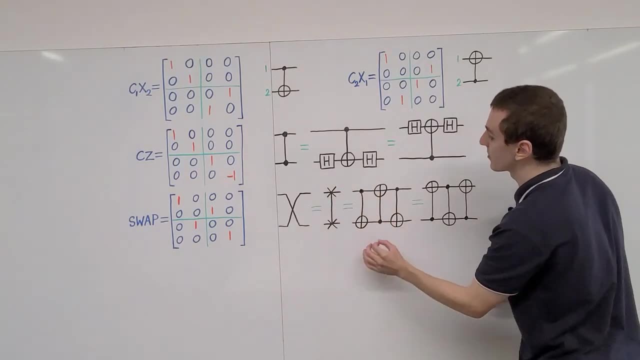 matrix and then a third matrix. But it is also important to remember the convention as to where you're going from. The convention in these diagrams is we go from left to right. So we would apply this matrix first, then this matrix, then this matrix, But for matrix. 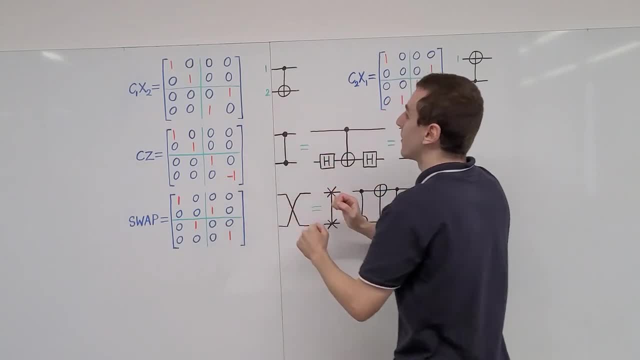 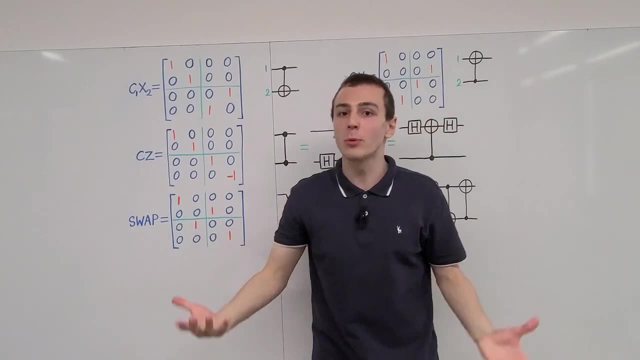 multiplication and applying on on these column vectors, we would have first applied the one that's furthest to the right and then the one that's the furthest to the left, And also we can use the associative property of matrix multiplication to collapse those matrix. 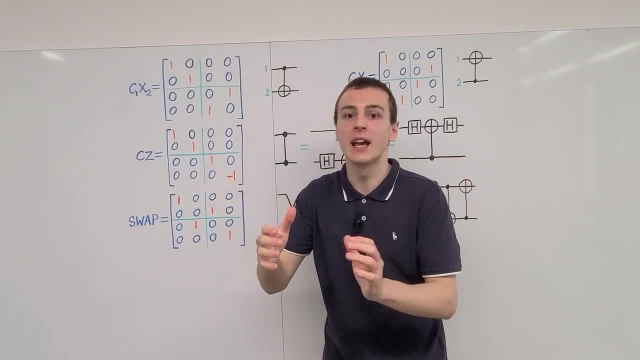 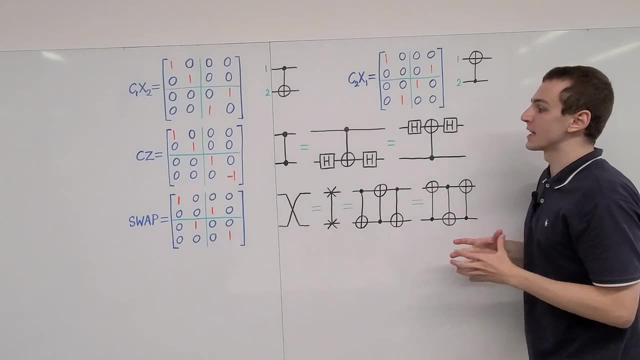 products together and we can just turn them into one big matrix and apply that onto the column vector. So now what we're going to do in the next video in the quantum mechanics playlist is have a look at where these matrix representations actually come from. We're 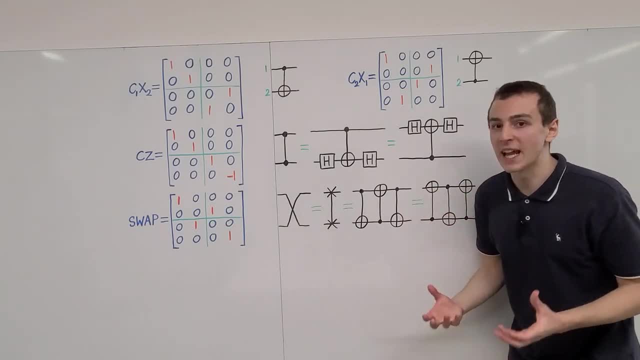 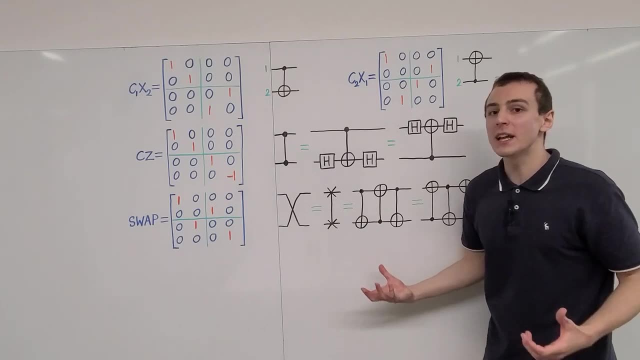 going to represent all of these matrices in terms of tensor products of the Pauli matrices, and we're going to see some very interesting properties. We're going to look at some inner products that emerge from the trace and we're also going to see why these circuit identities. 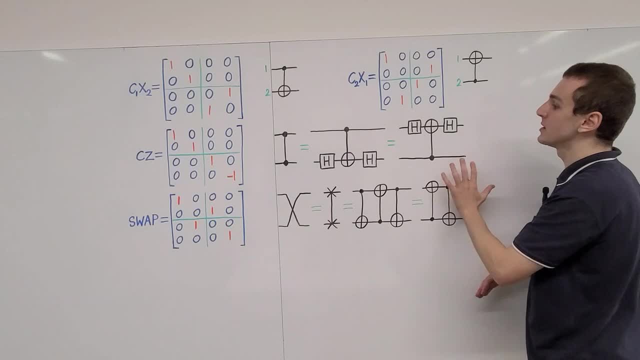 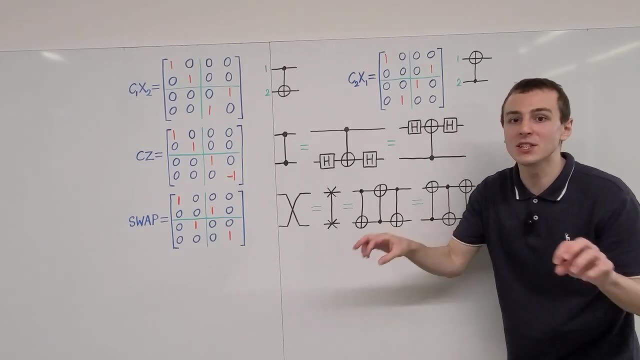 work. So these are visual depictions of what the matrices are doing and we will see. another way of looking at this is in terms of Dirac notation and writing down tensor products of matrices. So we're going to look at some very interesting properties and we're going to look at some 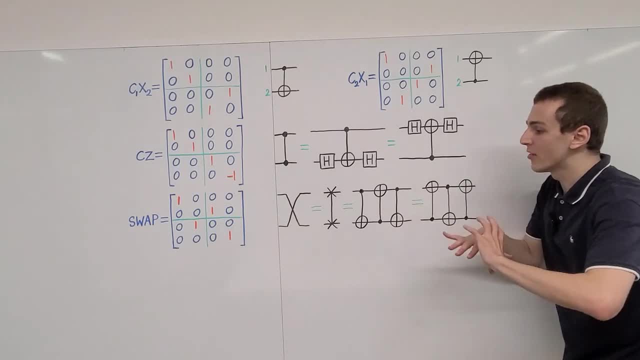 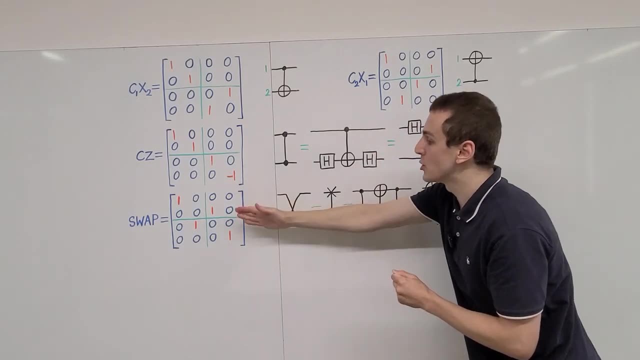 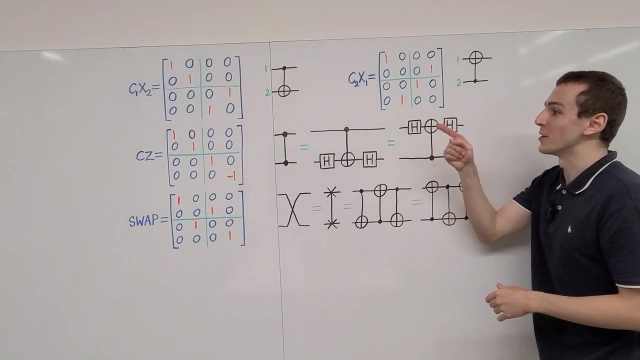 And these operators can just be written as letters, where we think of that letter as a general operator that can be represented either as a symbol or in its matrix representation. So you can find all the other videos in the quantum mechanics playlist if you click over here.